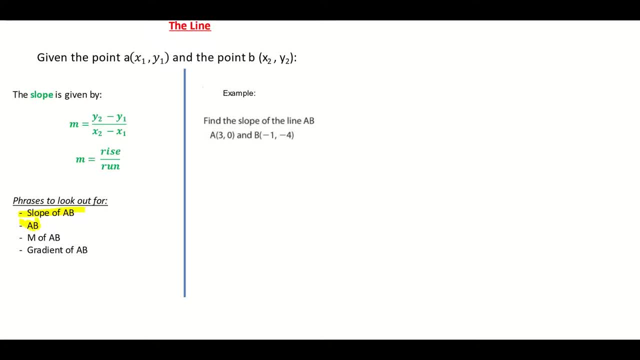 It could come up like this: find ab without the brackets. You'll also see in your log tables those modulus lines Finds around ab, which mean distance. so check another video for that. The letter we use for slope is m, so it might say find m, which relates to the slope, and another word for slope is the. 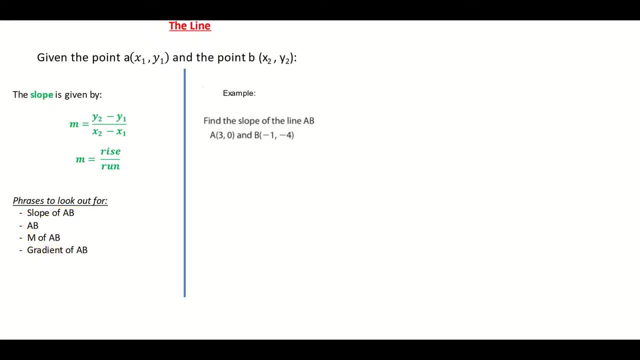 gradient. So they're just ways of writing the slope. Coming over to our example, here on the right hand side, I'm saying: find the slope of the line ab and I've given the two points a and b. Like any exam question we do, which involves a formula, we should always first of all write down. 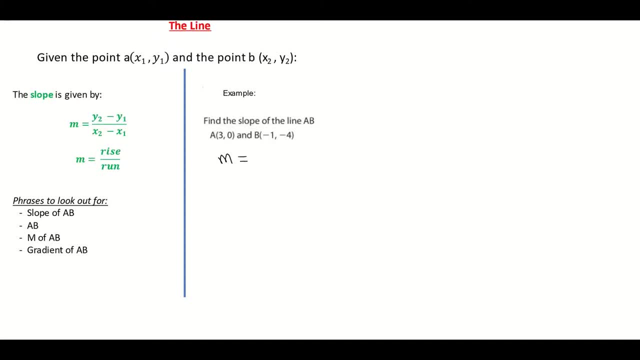 our formula. So my formula here is: slope, or m is equal to y2. take away y1 over x2. take away x1.. I'm then going to write down my two points before I sub them in, so my a and my b, and I'm going to label them x1- y1. 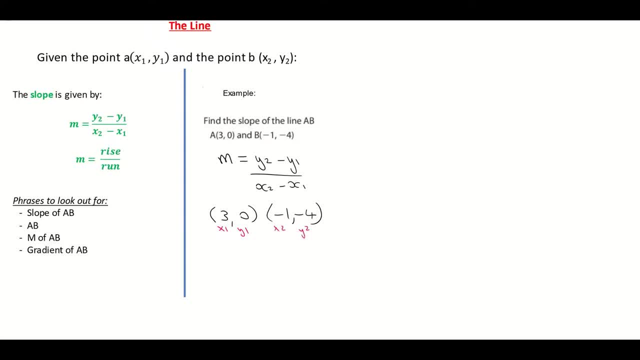 x2, y2.. So that's labeling the coordinates. I've also put down my formula. Now I'm going to sub my coordinates into my formula. so it's m is equal to first of all, and my y2 is minus 4. so I'm going to write down my minus 4. then the formula tells: 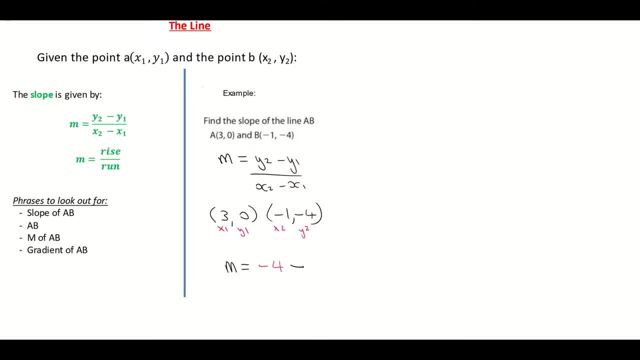 me to use my subtraction, so I'm going to subtract my y1. my y1 is 0, so I'm subtracting 0. that's all being divided by my x2, and the value of my x2 is negative 1. I'm then putting back in the minus from. 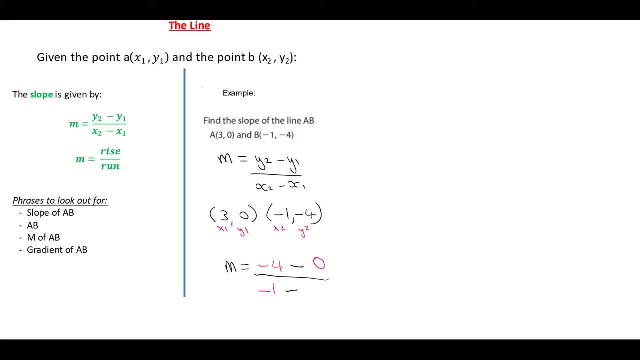 the formula and I'm now subtracting the value of my x1, and my x1 is a value of 3, so I'm subbing in my tree. I'm just going to make a bit of room here and bring it up to the right. so that is giving me. 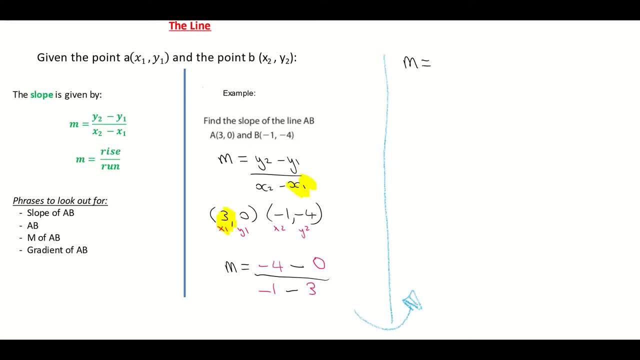 a slope of minus 4. take away 0, which is minus 4. I can basically just drop the 0 over minus 1. take away minus 3, so I'm on minus 1 on my number line and I'm going back. a further 3 units brings me back.